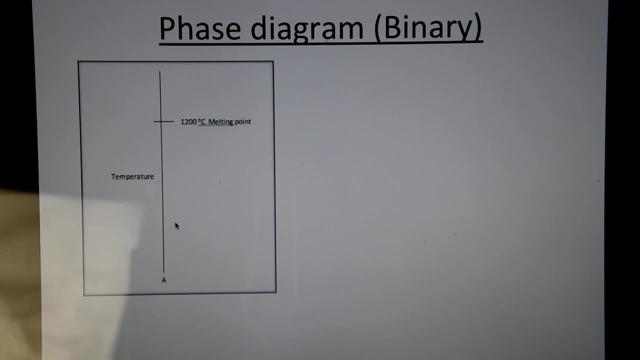 where the solid begins to turn into liquid. So for this example, maybe at 1,200 degrees Celsius the solid and liquid phase coexist within the microstructure. Now if you begin to introduce another element, for example in this case where we have B, then you don't just have one temperature. 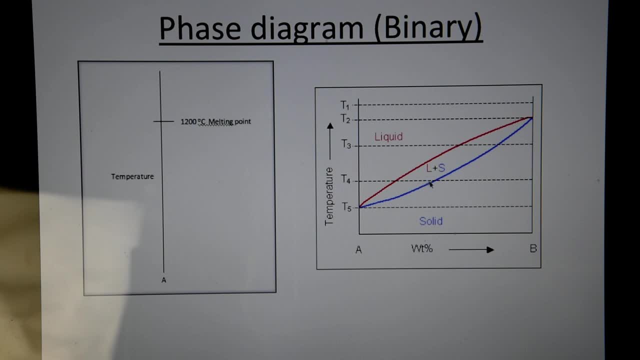 that exists within the microstructure. You would have a range of temperatures, as you can see here. So that's why we need to understand, with phase diagrams, what sort of phases are present. So you have a solid solution here: liquid and solid and then liquid. 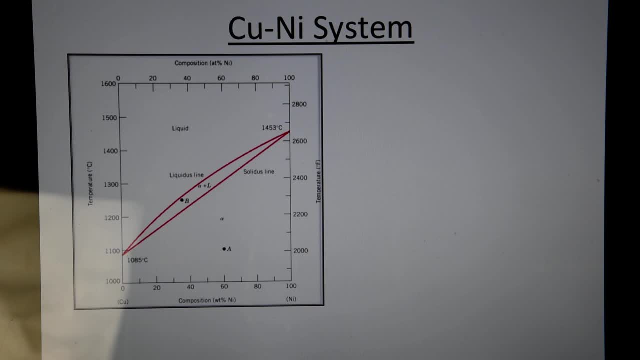 So now we'll talk about the copper- nickel system. As we saw earlier, copper and nickel are really close in the. when you look at the diagram I showed earlier, they're very close to each other. They have uniform or they have quite similar atomic structure. So, as you can see here, 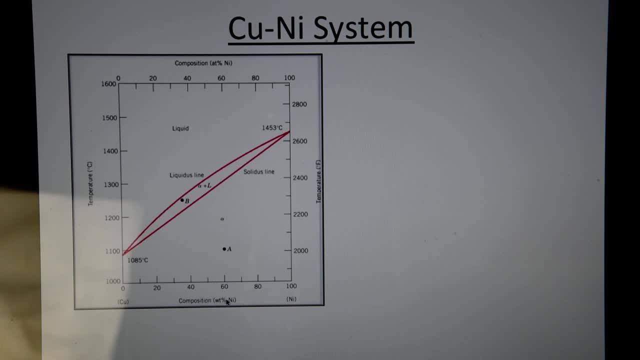 here, on this horizontal axis, you have the composition of nickel, which is called the weight percent of nickel. There are three main regions in this phase diagram. This region here, where you have point A, is called a solid solution and is denoted by alpha This: 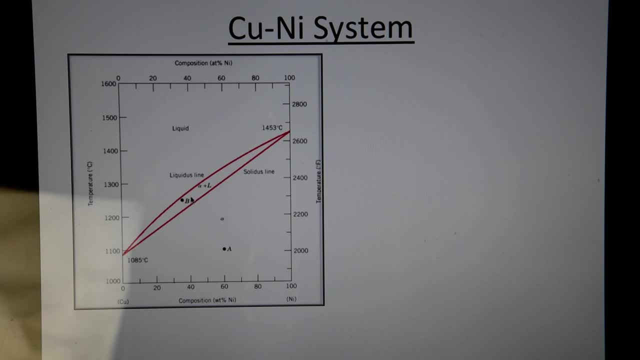 region in the middle here is called the alpha plus liquid, So it's both solid and liquid. This is where the melting is taking place, And above here is called the liquid region. And this line here which separates the alpha region from the alpha plus liquid is known. 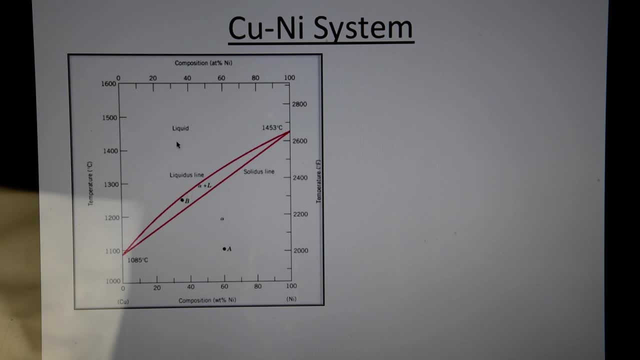 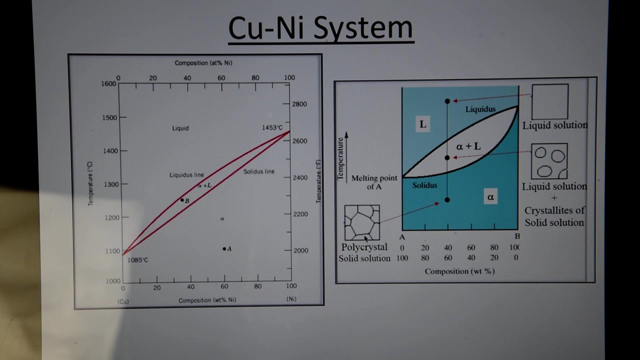 as the solidus line, And this line here, which separates the liquid region from alpha plus liquid, is known as the liquidus line. Now, if you look at the microstructure which is present here, during the solid solution, you've got grains and grain boundaries. Now, if you move to the alpha plus liquid region, 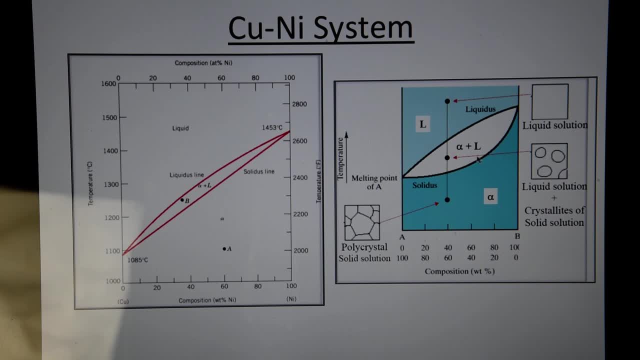 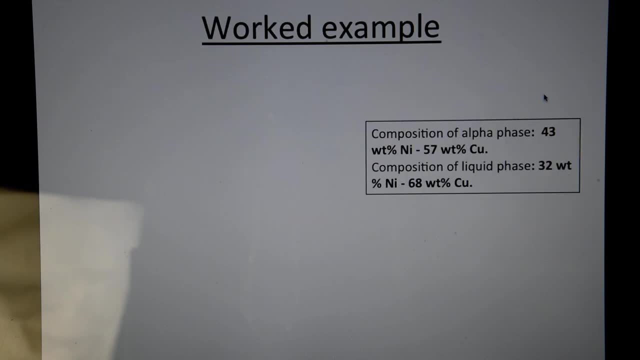 then liquid begins to form. That's shown by the empty space And when you go above that region into this phase, it's just liquid which is shown by this empty box. Now I'll go through a record example just to help you understand liver rule and its. 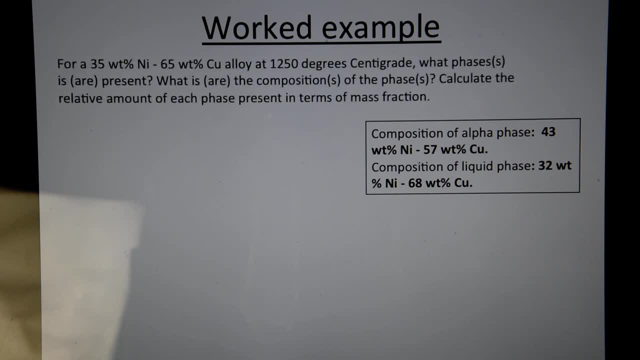 high line. Now this question says you have 35 weight percent of nickel, which is the same as 65 percent weight of copper, And this is at 1250 degrees Celsius or degrees centigrade. The question is asking: what is the weight percent of nickel and what is the weight percent? 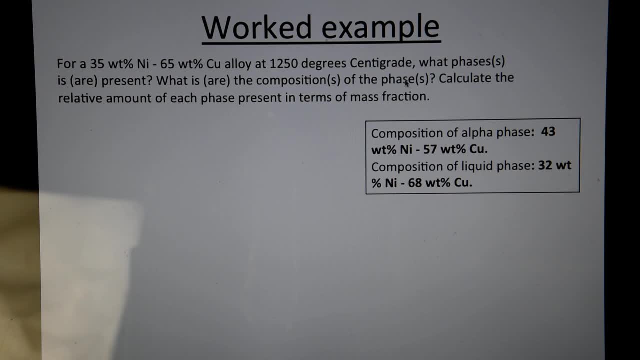 of copper. The question is asking how many phases are present, or what phase is present, What is or are the compositions of the phase, And calculate the weight percent or the mass fraction. Now, to start with, this is an expanded image of the copper-nickel phase diagram. What you 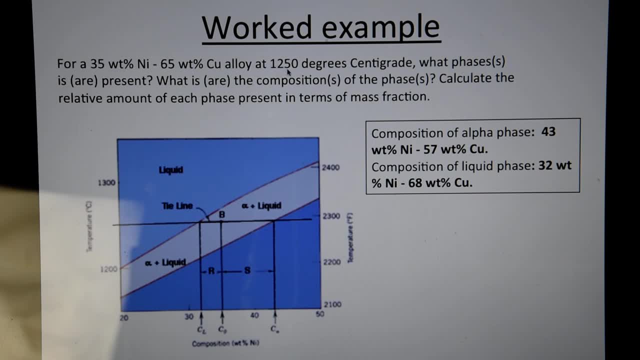 have to do first is take note of this temperature: 1250 degrees Celsius. You have to draw a horizontal line here. 1250 degrees Celsius. You have to draw a horizontal line here which intersects the liquidous line and the solidus. 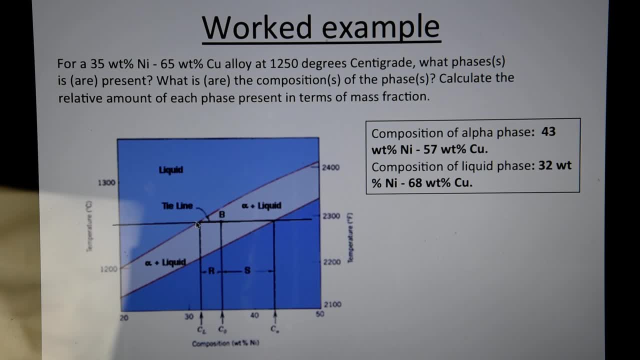 line. This line is called a tie line. Now, from there you project down. So whatever point you've got here, just project it down and that gives you the composition of the liquid And the intersection here. if you project it down to a horizontal axis, it gives. 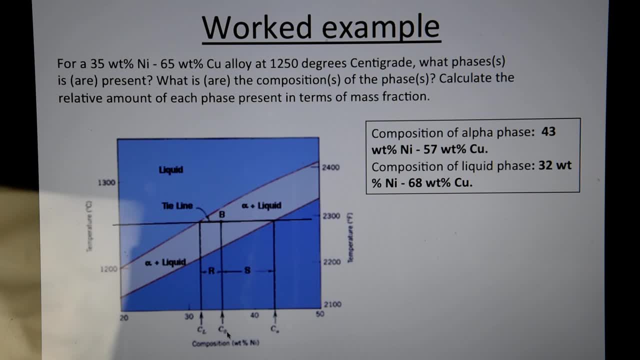 you composition of alpha. You have your original composition here, which is given as 35 weight percent of nickel. So, first of all, to answer the first question: what is the weight percent of nickel? You have to know. First of all, to answer the first question, there are two phases present because we are 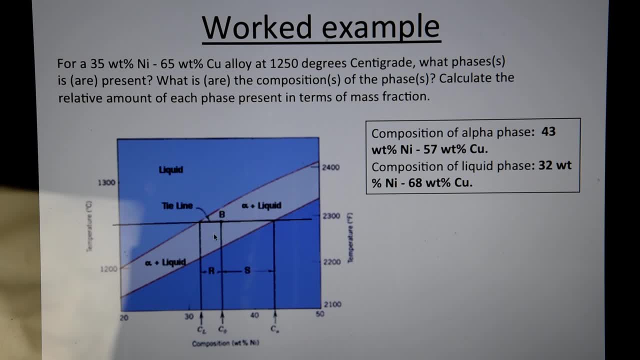 in the alpha plus liquid phase region. Now, second is asking us what is the composition of the phases? So C alpha is approximately 43% nickel and C liquid, which is the composition of liquid, is 32% nickel approximately, And this also translates to 68% of copper And this also translates to 68% of copper. Now to answer the first question, there are two phases present. So how many phases are there? 30,000.. And this is the composition of the phases. Now the question on the right. 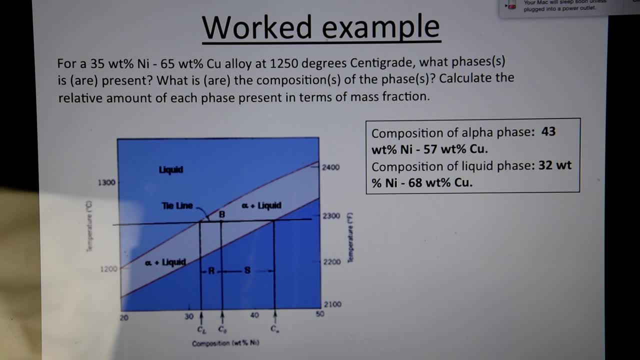 one has a friend of mine who has been working in the pump field here for 30 years. He has been. The third part of the question is asking us to find the weight percent or the mass fraction. To calculate that W alpha, you need to take this value here: R over R plus S.